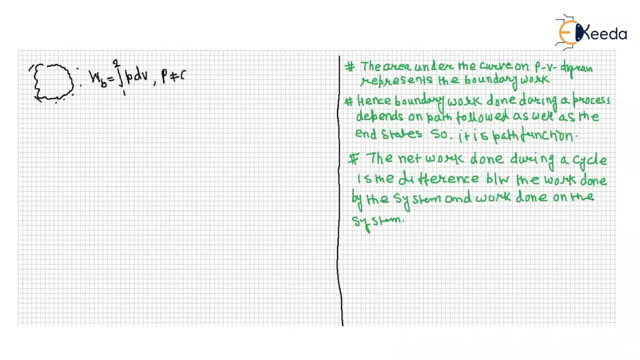 And mind it, p is not constant, The integration only evaluated if p is the function of d- g. Right Now, in this section, we will discuss about how to represent this work on p d diagram. See, this is your thermodynamic plane. 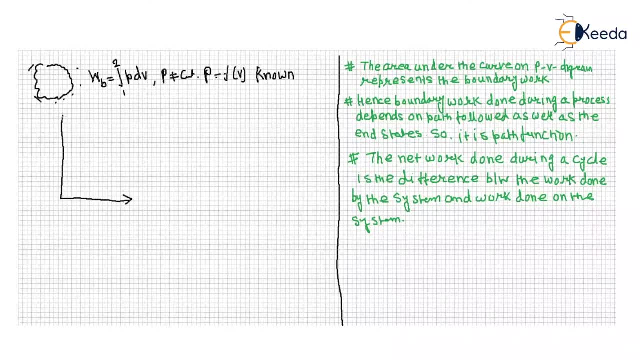 Let's suppose that this is your p, d and g Right? If you know about the initial system pressure, it is at the stage 1, p1 and g1.. After its expansion of the system boundary, the pressure will reduce and volume will increase. 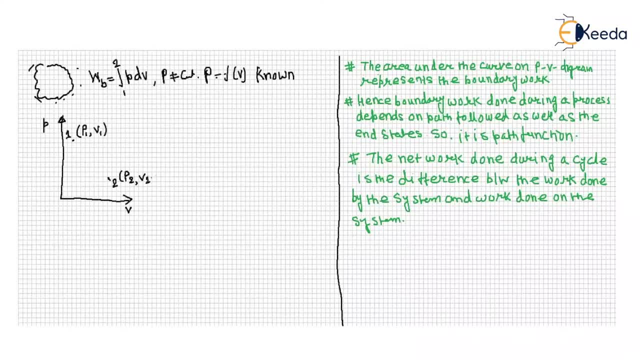 Let's suppose p2 and b2.. And due to its quasi-equilibrium, static manner, then you join this process by a path, Right? So this is your process path If you project the process 1 to 2 on a volume at which- let's suppose d1 and there is a volume d2.. 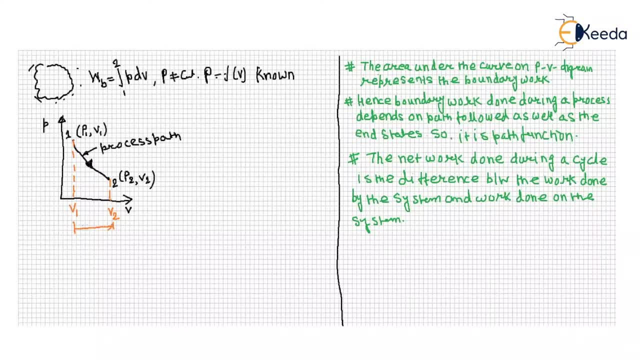 And this is your change in volume: dv, Right. Let's suppose there is a cylinder has a total volume v2 and its initial volume v1.. And the piston will move in between v1 and v2.. Let's suppose this is at any instant of the piston. 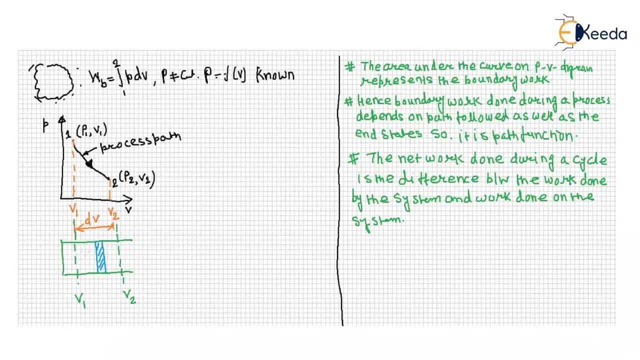 There is a simple, compressible substance which is always exerts a pressure. Why? Because expansion of a boundary p. So if there is a displacement is the displacement of the piston. let's suppose this is a displacement of a piston dv. This is a displacement. 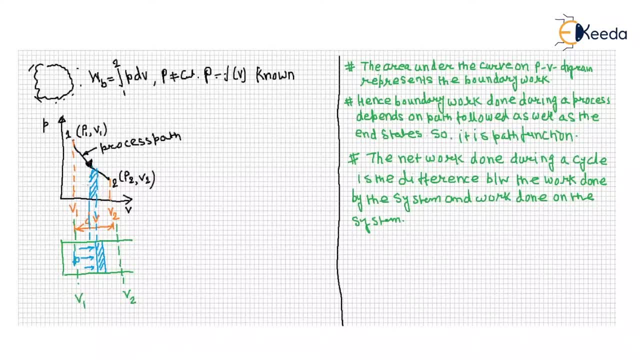 Right. So what is the area of this graph? dA is equal to p into dv and the total area from 1 to 2. integrate this total area from 1 to 2 dA. that means integrate 1 to 2 p, dv. 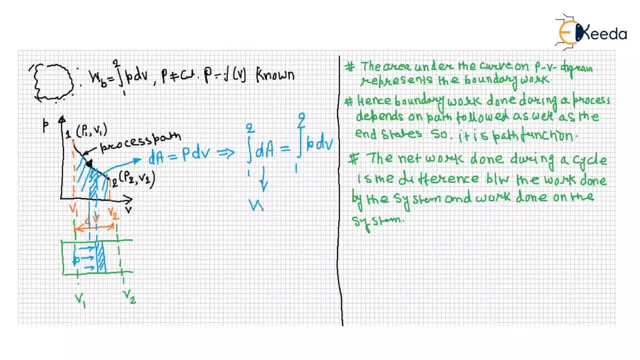 then this is nothing. This is your boundary work: 1 to 2, p, dv Right. So p dv, p into dv is the integration over 1 to 2 which give indirectly total area projected on a volume axis. That means, if you find the work transferred, 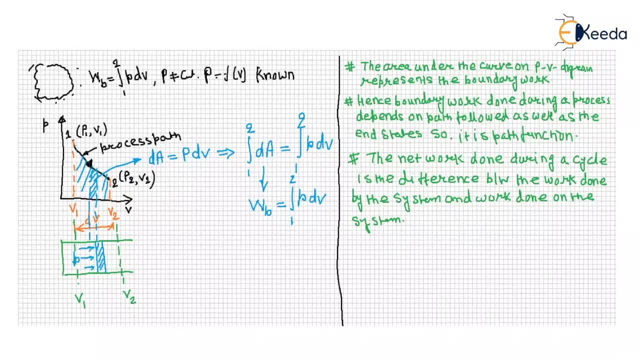 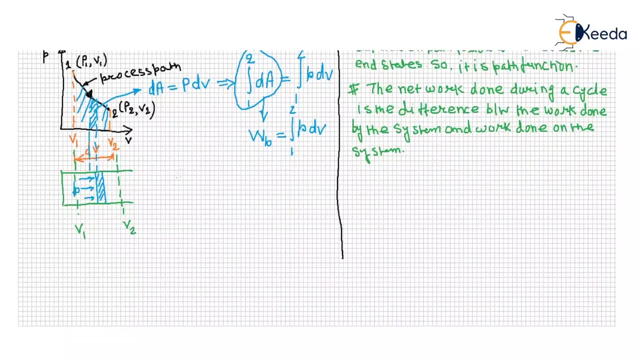 by the system during a process 1 to 2. just you integrate the area under the curve on volume axis from 1 to 2, then this gives the boundary work Right. See, if this is our pressure and volume diagram. there is one point, p1, and 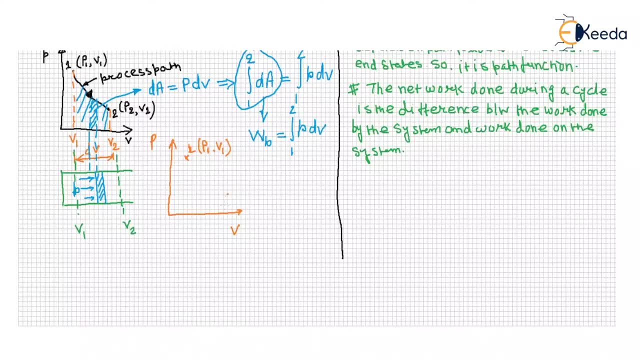 d1 after expansion. there is a second point: p2 and v2. there is v1, there is v2. there is pressure p1, there is pressure p2 and if you join by this process from 1 to 2, p1, there is a pressure. 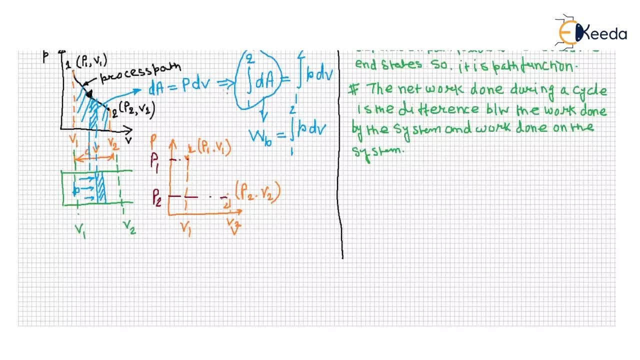 p2, and if you join by this process from 1 to 2, p1 to 2 via part a and with other process, 1 to 2 via part b and one another process join 1 to 2 via part c. so the area 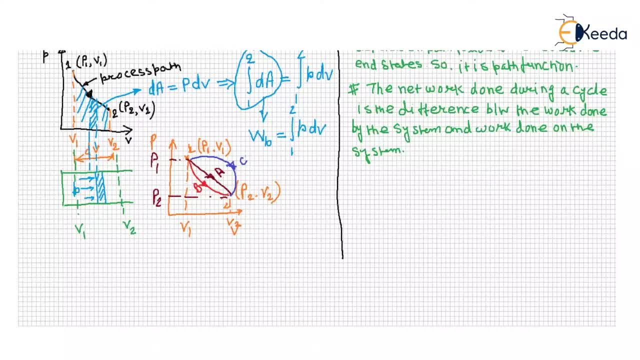 under the curve is 1 to 2 and the area under the curve on volume axis. the area under the curve on volume axis is this much and the area under the curve on volume axis of the pressure b is same but there is different, different part, the area. 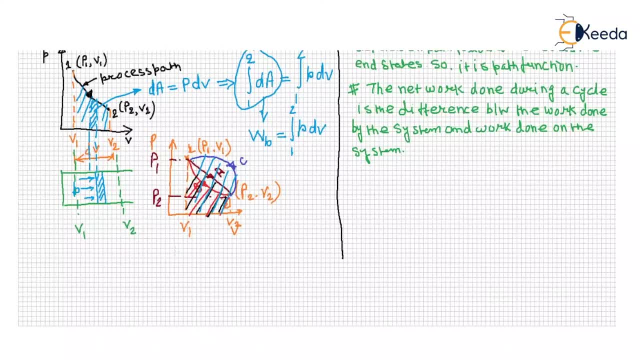 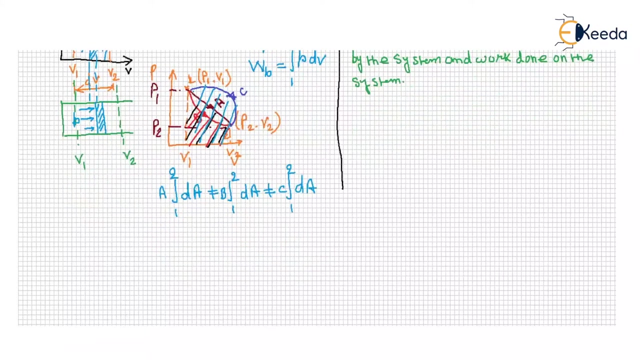 will differ. that means integration 1 to 2 of area d a via part a is not equal to integration 1 to 2 of area d a via part c. so boundary work via part a is not equal to boundary work via part b is not. 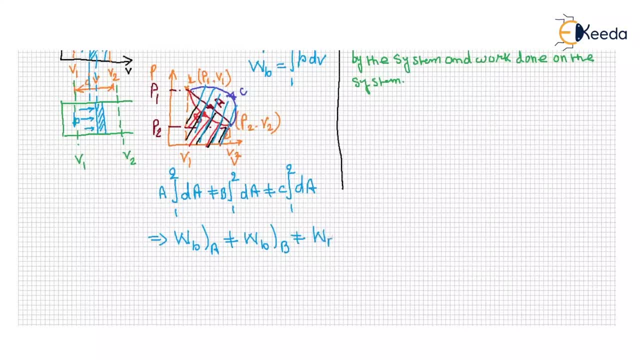 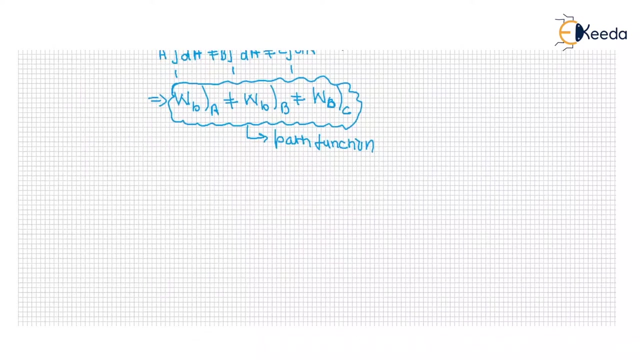 equal to boundary work via part c. so this is a path function. this is your path function, right? if you find? let us suppose there is a cyclic process which is a path function. so if you define a cyclic process on easy diagram e and v, you know that. 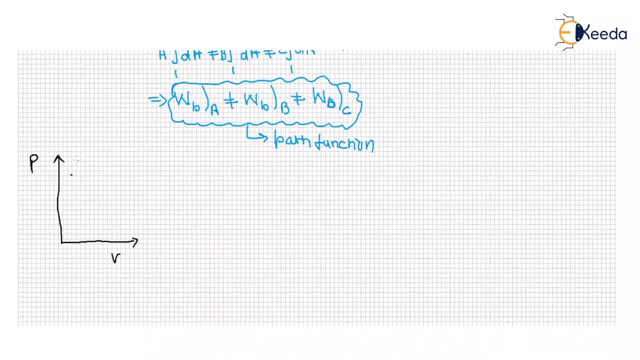 already the minimum number of process to define a cycle is 2. that means 2 is at 1 via path a, and if this is cycle, then 2 is at 1 via path b. so what is the area under the curve via path a, via 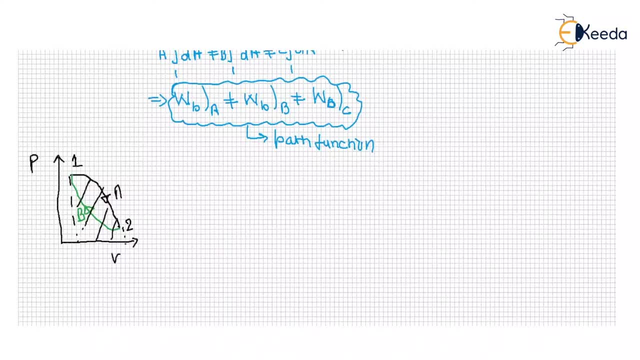 path a and via path b. this is your area, so the net is this is your w net. that means the net work during a cycle. net during a cycle is the work done by the system minus work done on the system. these two differentiation differentiate with the network. 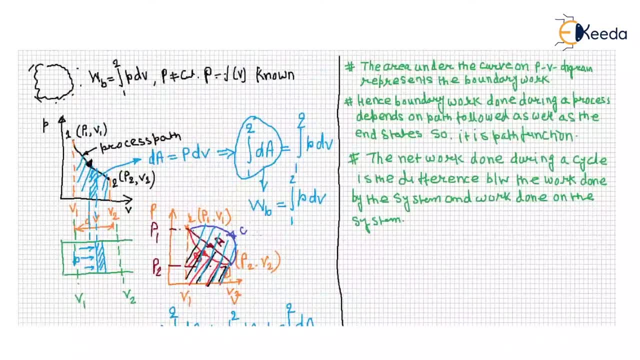 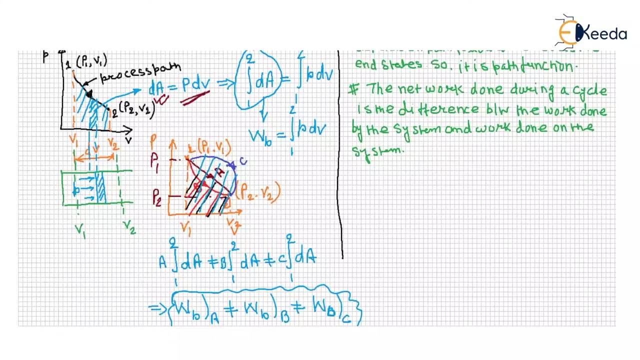 right. so there is some facts about. the curve on pv diagram represents the boundary work. that means what is the area under the curve on the volume axis is a representation of boundary work. number second is the end state. so it is path function. see boundary work depends on the 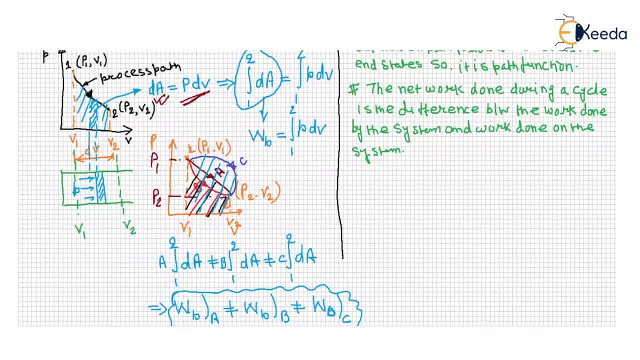 path followed and as well as end state. so it is a path function. why? because each and every path, there is a path function and it is a path function which is a path function and this is the path function. so this is a path function which goes to. 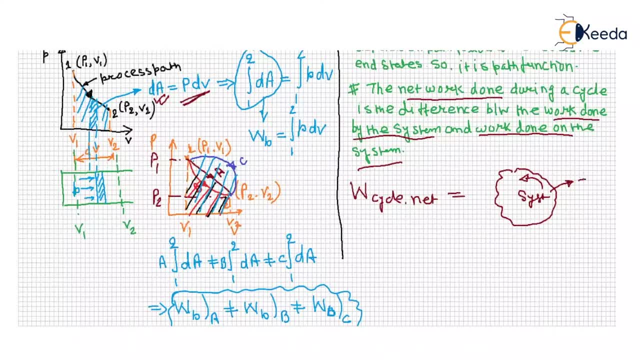 develop a work, then work is positive. if the system work done on the system, the work is negative. so the difference of these two work and network all the way is the differentiation of word done by the system minus word done on the system. right, work done by the system. let's 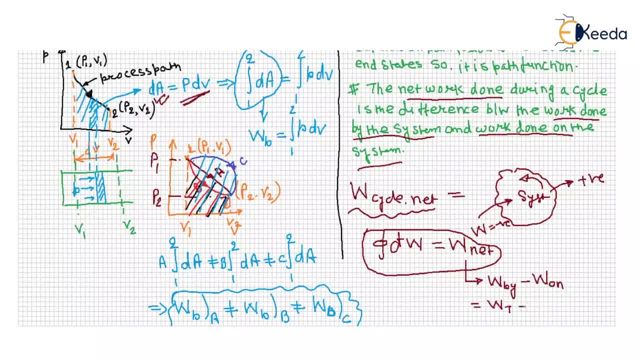 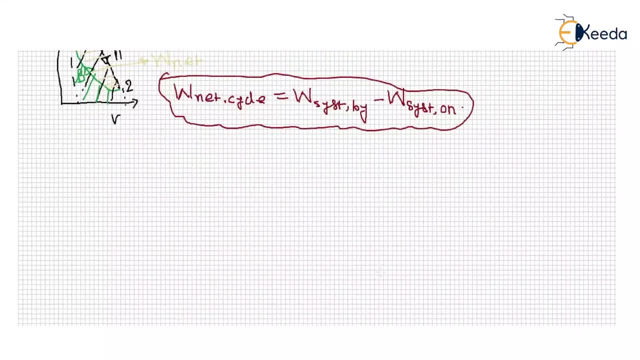 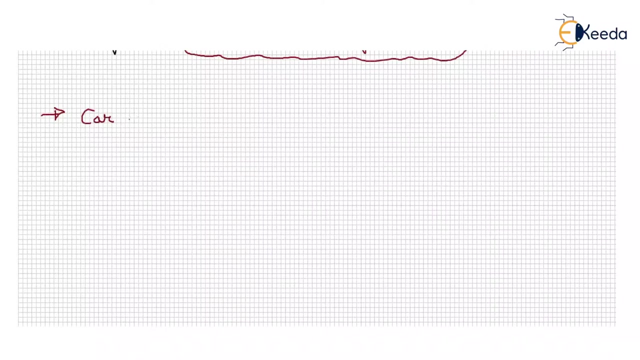 suppose WP and work done on the system. let's suppose WC. so this is your net work done during a cycle. another aspect is that let's suppose there is a car, engine, engine in which there is a piston, and this is your cylinder, this is your cylinder and this is your piston, connected with a connecting. 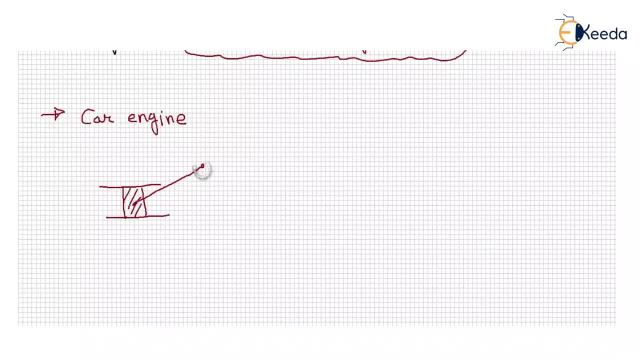 robot and this connecting rod is connected with a crank and this crank is connected with a crank shaft, with a crank shaft, and this is your piston, if we develop a power to derive the crank shaft. if, in this condition, what is the boundary work? the boundary work is the summation of 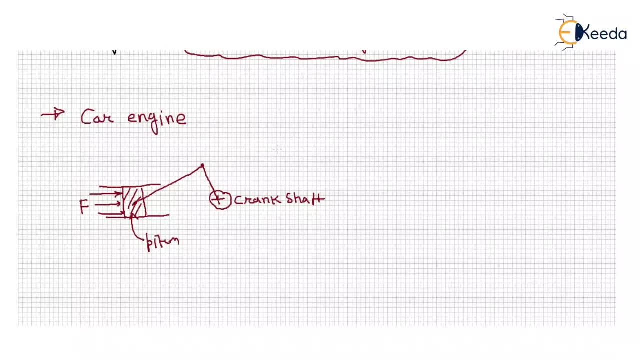 energy transfer by the system and work must be equal to the energy received received by crank shaft, energy received by a crank shaft and the atmospheric pressure and the energy used to overcome why? because there is a piston cylinder arrangement, there may be a friction, one connecting rod, a crank shaft, there is a crank, there is a rubbing between that and 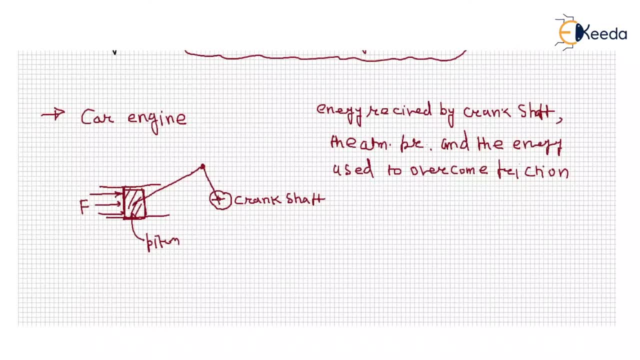 their crank and their shaft is rubbing between that to all accounts with the friction and this will overcome to the friction. so in this system, what is the boundary work? the boundary work is that work overcome due to friction. just add all of this work done against atmosphere plus by the cause engine run against a system. 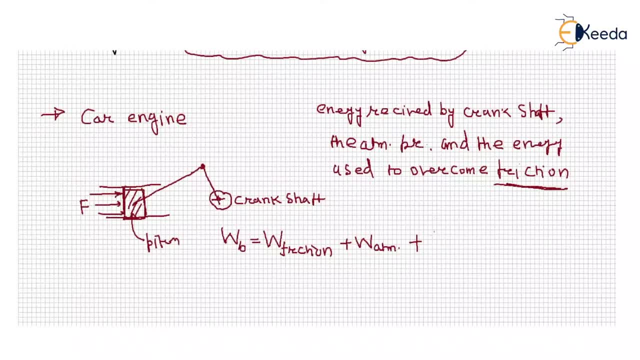 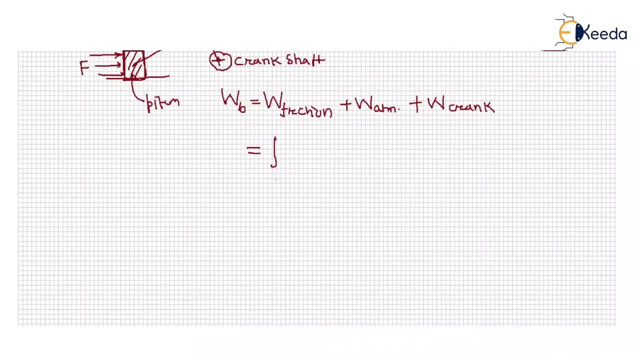 then run against a system, scope and work received by the sound. so if we integrate from one to two force due to friction plus, what is the atmospheric force? p, APM into a is the atmospheric pressure plus work force received by the crank into this is your atmospheric force, this is your friction force and this is your. 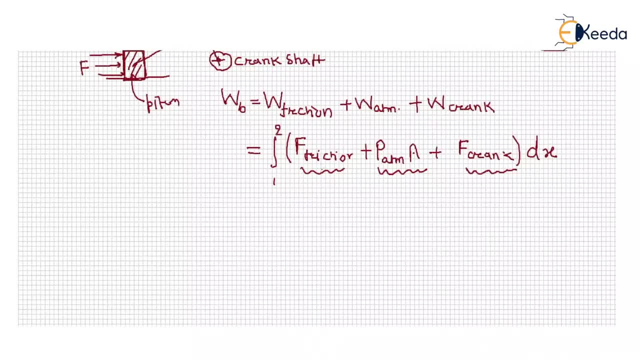 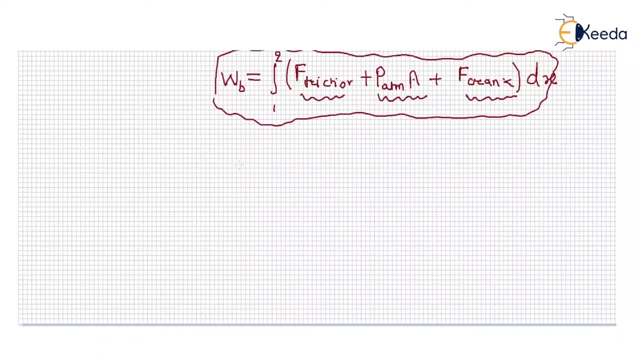 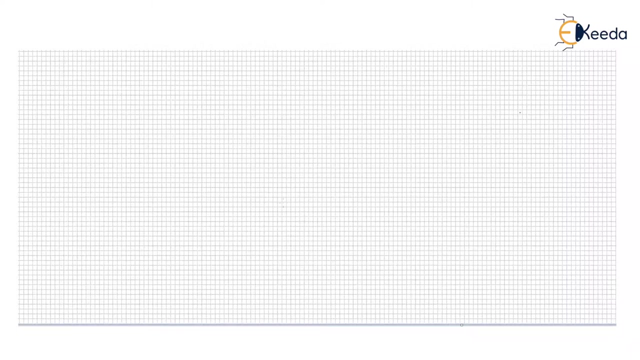 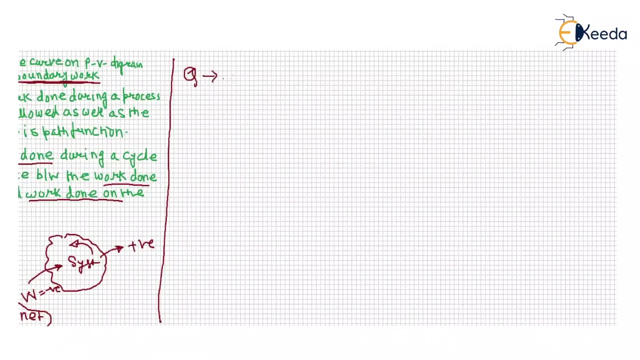 work force received by the crank. if you integrate 1 to 2 with a, d, x, then you get one rival during the movement of a star engine. again, one very important question in our mind is that very important question in our mind is that it's a question why this? 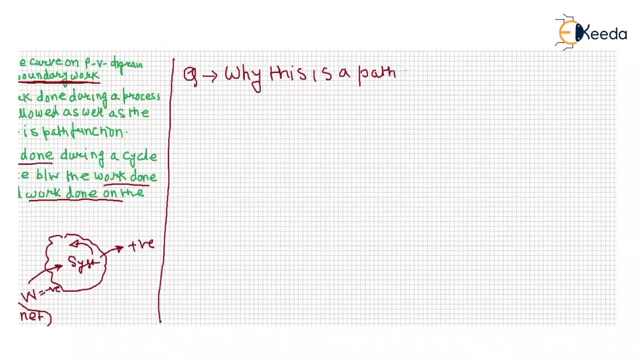 is a path function. that means why the boundary word is the path one. if someone asks you intuition, intuitively, then your answer is that sometimes in yes, there are two mark question always ask like that in es: examples: right, depending upon upon how the pressure, how the pressure changing with. 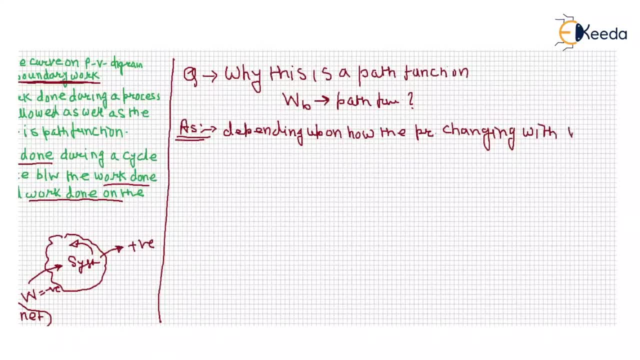 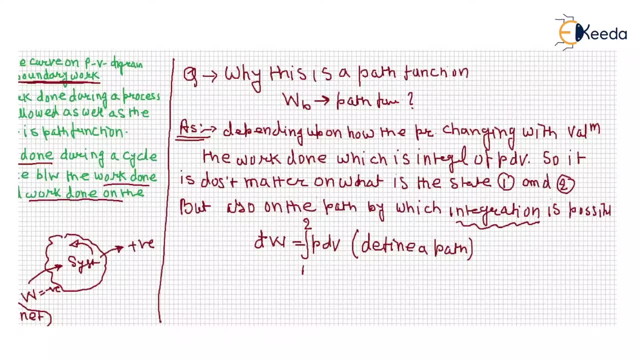 volume, the work done with the pressure, which is integral of p, dv, right, so it does not. it is does not matter on what is the step, is the state one and two, but also on the path by which integration is possible. why? because integration is possible, you, you. 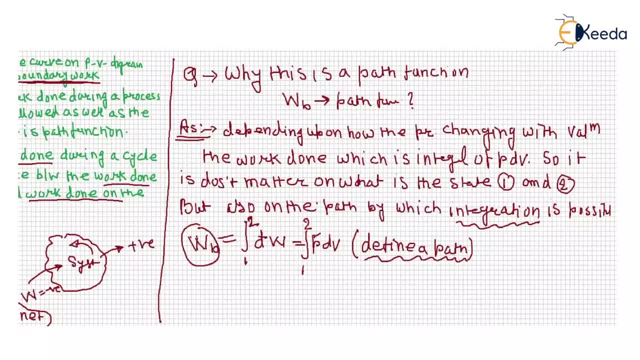 you must be no initial and final point. that means if p is the function of volume into dv, if you solve it not only from one point to two point but also apply integration. when you apply a integration to find the total boundary work, you must be follow a path. 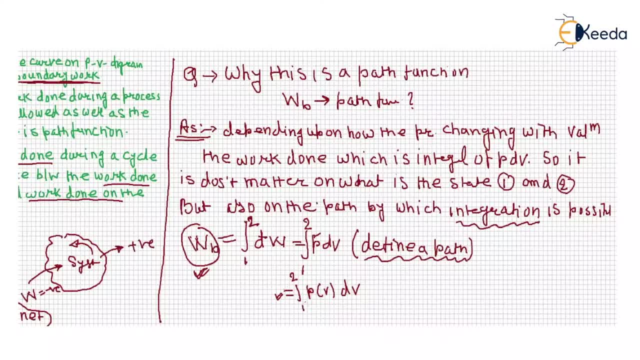 without define, defining a path, you can never achieve integration of dvd. so to evaluate the boundary work, you must know about path, not just only you know about the in the condition, not, it is sufficient- also defined a path. so boundary work is a path, function now one, very, very. 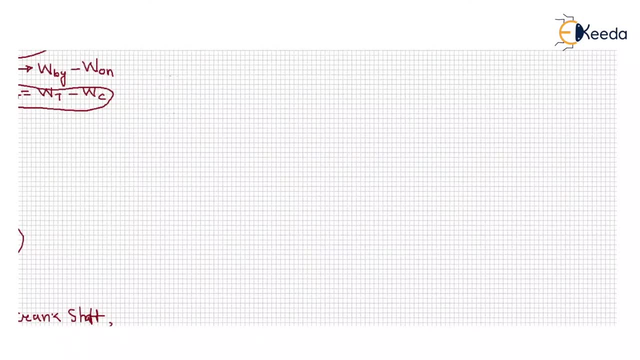 important observation. see, my dear student, lots of book. there is a confusion and if you see about many youtube channel, there is a big confusion, creates a big confusion and clearly clarify that confusion. see, there is necessarily that boundary work or displacement work work has to, has to be a closed system.